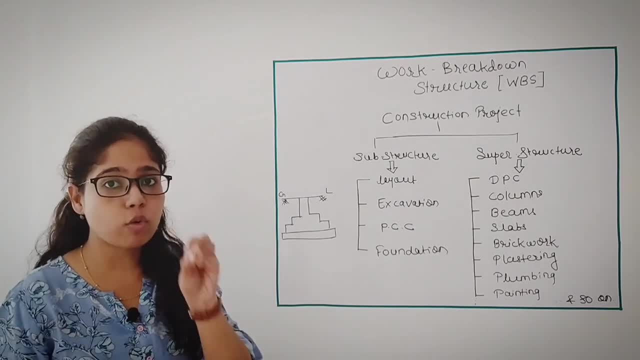 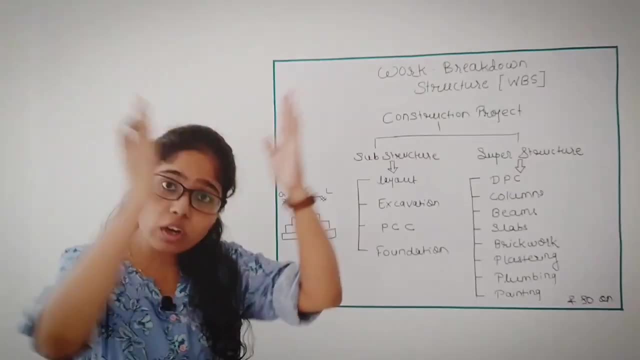 have to divide into sub activities so that you can focus on each activity. So let us take an example. Suppose I have one construction project. Now that whole construction project I have divided into two sub parts, that is, substructure and superstructure. Now, when 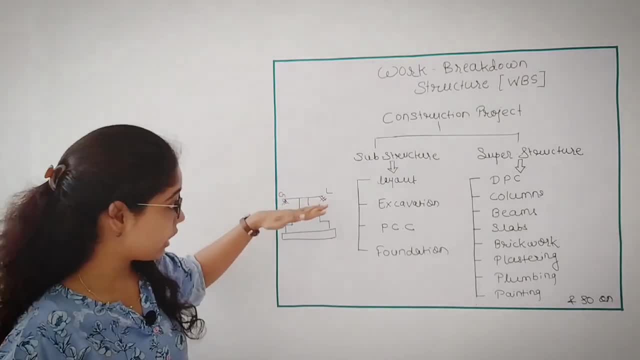 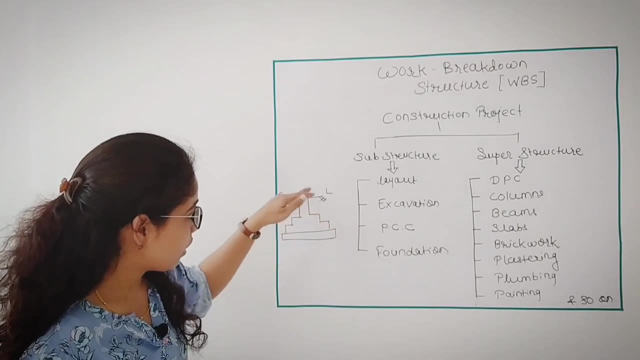 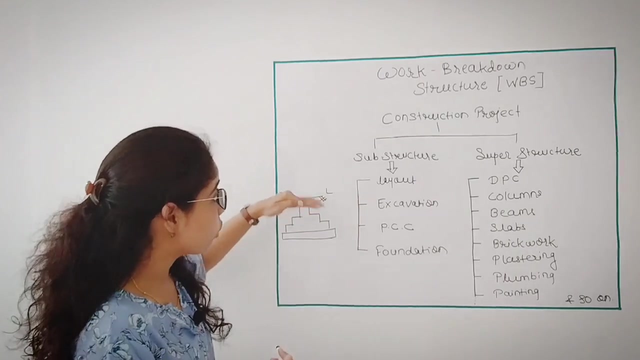 you call a structure as substructure, if the activities of the project are below the ground level, see the ground level. this is your ground level and below the activities of ground level That will be categorized under your substructure and the activities above the ground level. 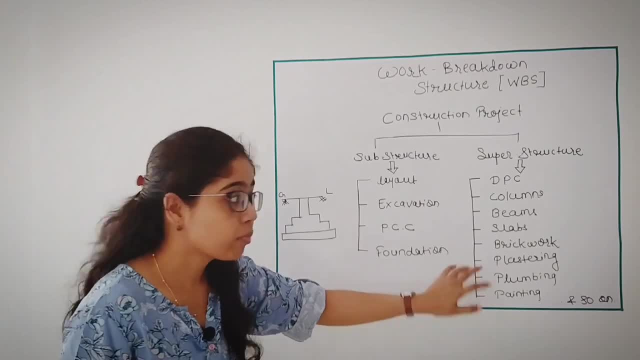 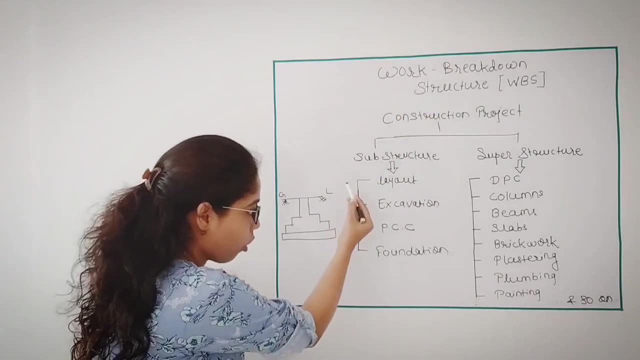 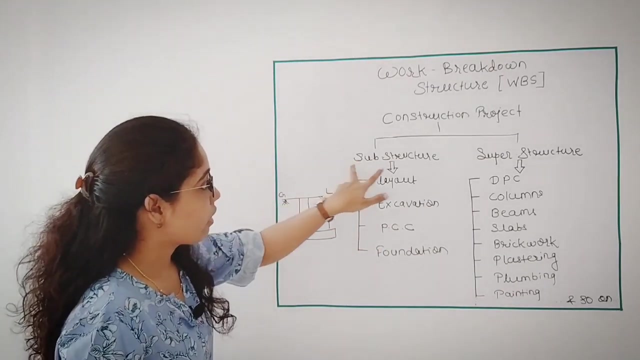 Okay, so these are the activities which are above the ground level that you have to categorize under superstructure. Now WBS will help you to divide all those projects, all that particular project, into number of activities. Likewise, like you can see, I have divided this substructure. 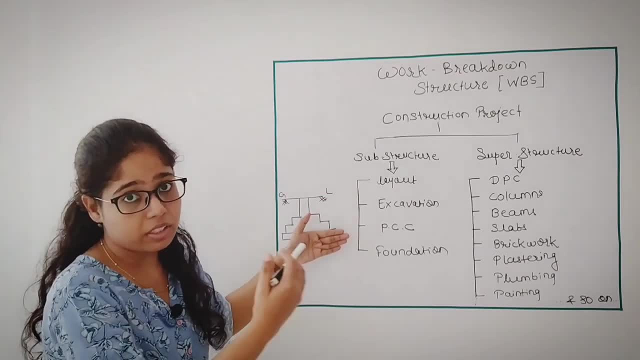 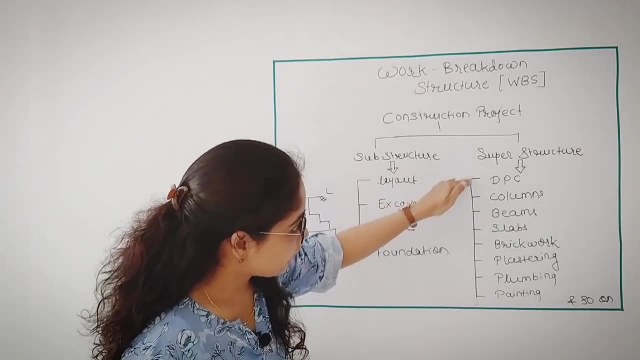 into number of activities. Whatever the activities comes under your construction, that will be categorized under your substructure. Now WBS will help you to divide all those activities into number of activities, Like, if I take, for example, superstructure Politics, I have divided it further and here in superstructure I have divided whatever the activities comes. 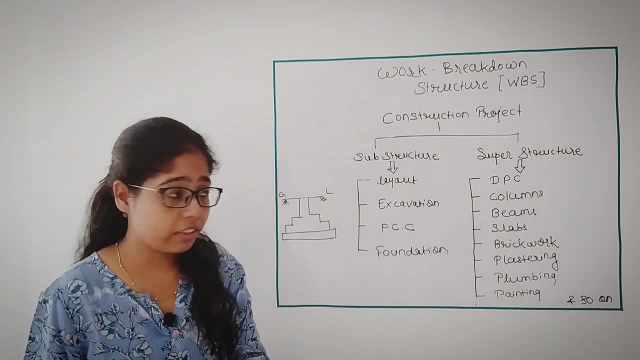 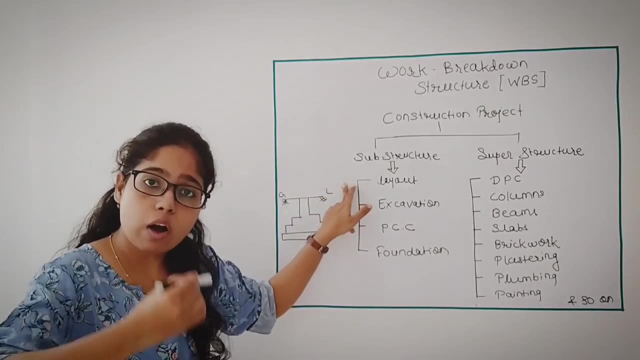 under superstructure. So first you have to divide the activities. Now next task is you can focus on each activity Like first activity is your layout under substructure and then your first activity is your layout. Now how you can focus on that and for particular layout. 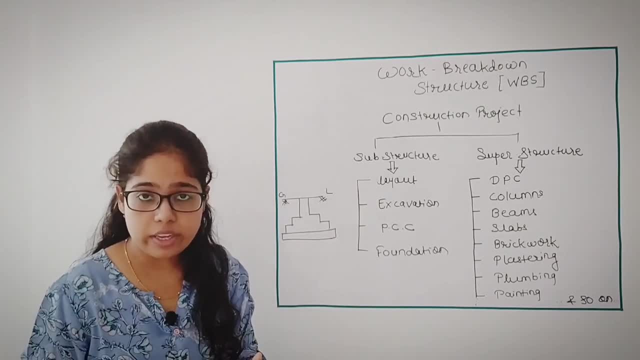 you should have the drawings, measurement drawings. They all have their size, and then all active activities should be there. Now, here, here is the mix up on less activities. Now I wanted to talk. that is what we call as Measures By, Measures in Measures. this plane will give you the choices Here. the Resident here means the layout. First activity is Constructed by Nope. 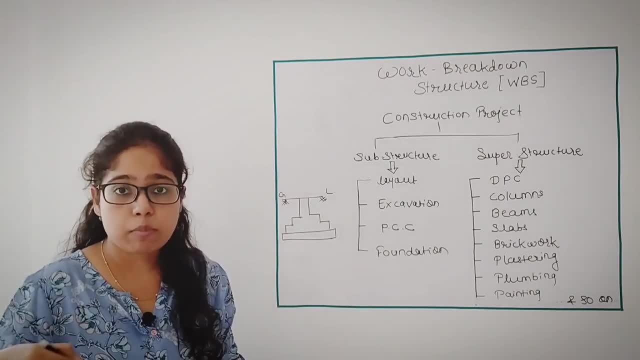 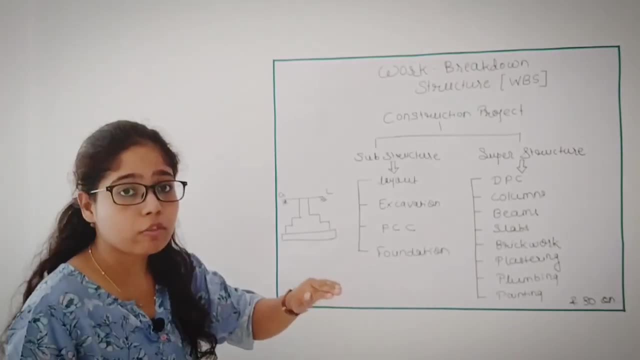 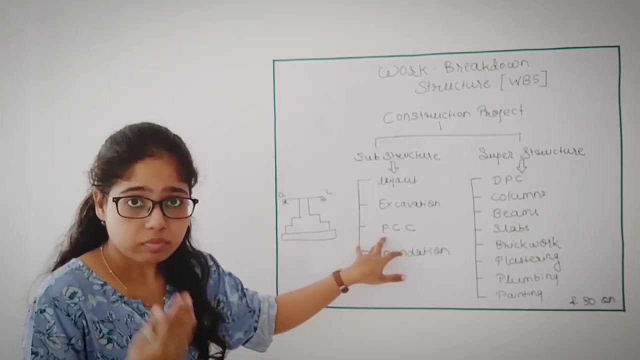 then only you can draw the layouts with the help of chalk. next is your excavation. once you done with the sizing, that is layout the next you can focus on excavation. once you excavate, then first part is PCC. now for PCC. whatever the data you will require, like again, you will require drawing. then for PCC: 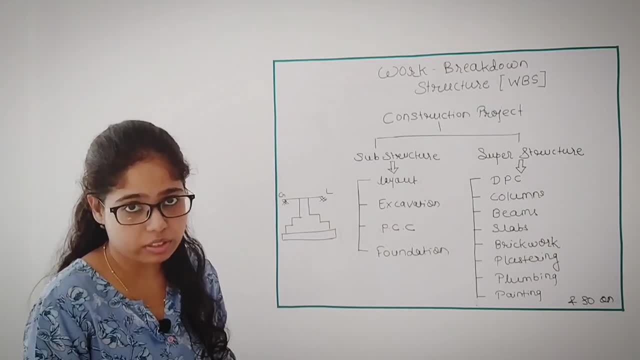 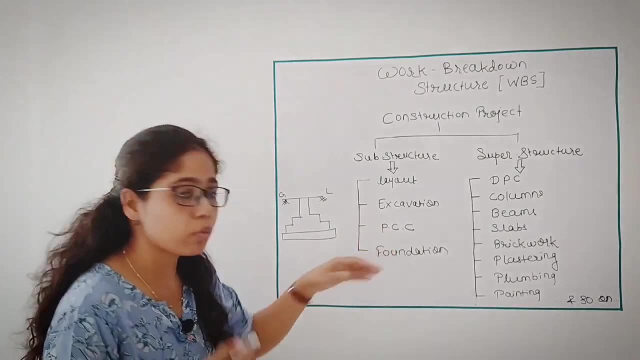 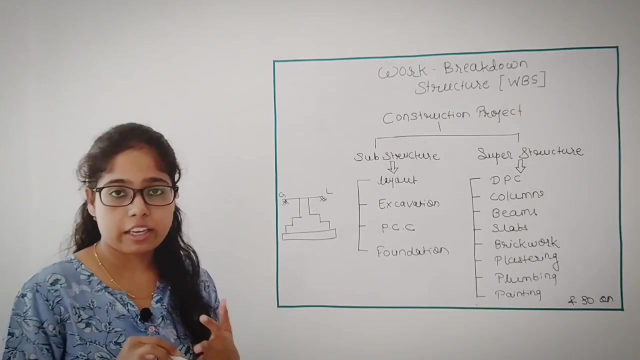 which type of concrete mix design you are using. that is M30, M40. so likewise you can focus on each activity. now for PCC, what will I get like which concrete mix I want to make? what will I get for that? I have to see that. so what happens in WBS? I can focus on every activity.